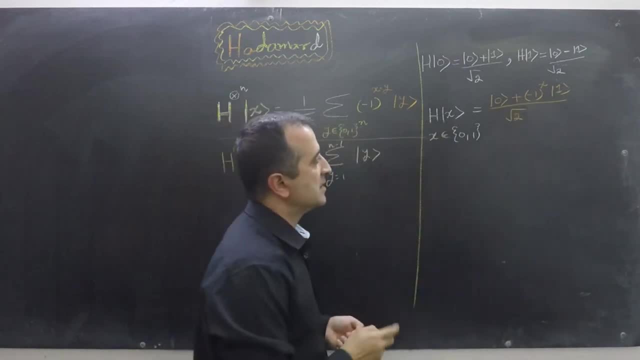 ket 1 raised to power x works because we know that the sign is minus in case of 1 and sign is plus in case of ket 0. So when we say minus 1 raised to power 0, then it becomes 1, so 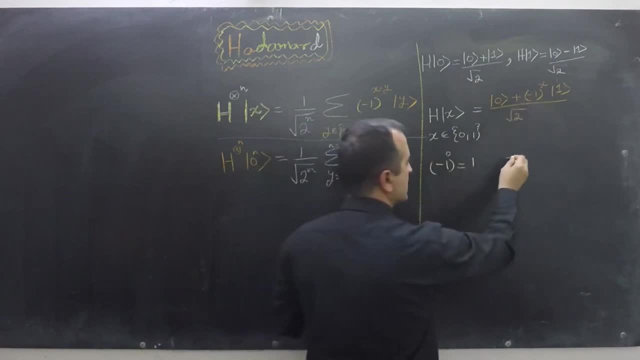 the sign remains plus. When we say minus 1 raised to power 1, then in that case answer is minus 1, so the sign changes to minus from plus. So that's why this formula works in both of those cases. But now we have to make this formula even more general by using summation. 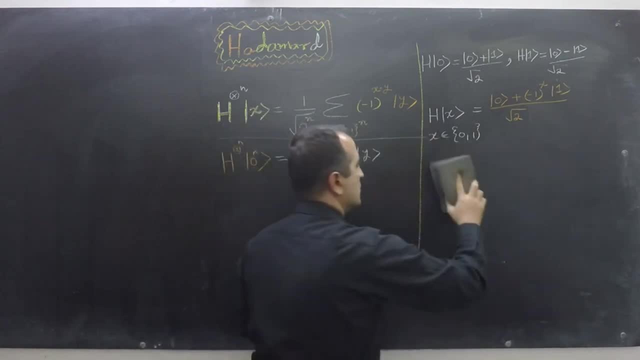 sign. So we say that Hadamard gate being applied on ket x, where x could be either 0 and 1, is equal to summation, And for summation we have to introduce a new variable, because that variable should take value of 0 and 1.. X could be either. 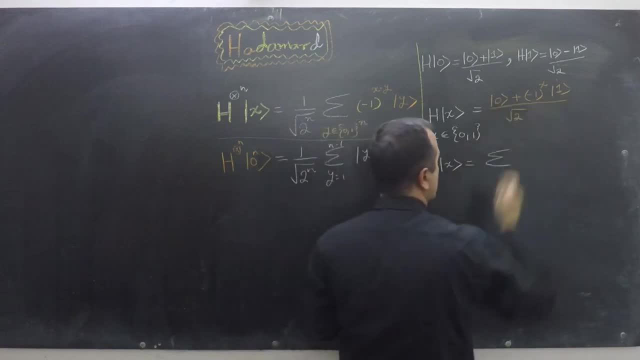 0 and 1, but the variable should take both values, first 0 and then 1.. And there are different ways to write summation. One way is that you can say new variable y, and y could take value from 0 to 1.. And this way of writing summation also works, but mostly. 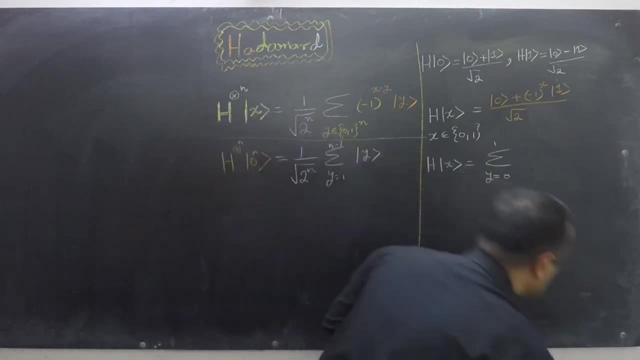 people don't use that in quantum computing. Mostly people use this way of writing summation that they say that a new variable, y and y, belongs to 0 and 1. And then to here we have to get y, because first y will take value of 0 and then y will. 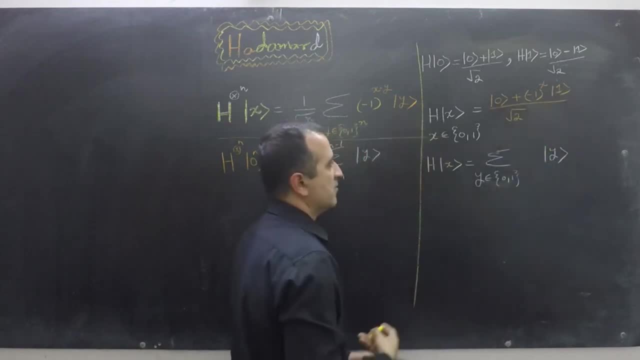 take value of 1.. Obviously we have to also write 1 overwritten. Now the only thing left is the sine. Here sine is rms positive with 0, ket 0, but with ket 1, sine will be a minus. a sine could be plus. So we write here: minus 1 raised. 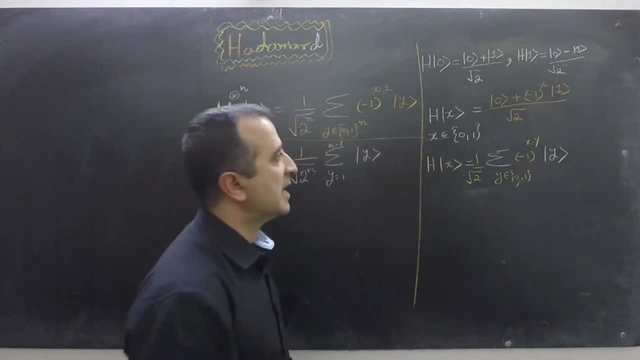 to power x dot y. It is because sine is minus 1. when we have this x here 1, and this y here 1. Then sine should be minus 1.. So that's why we say x and y, So the sine will. 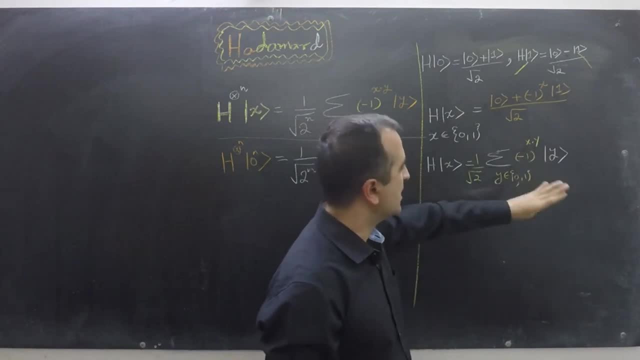 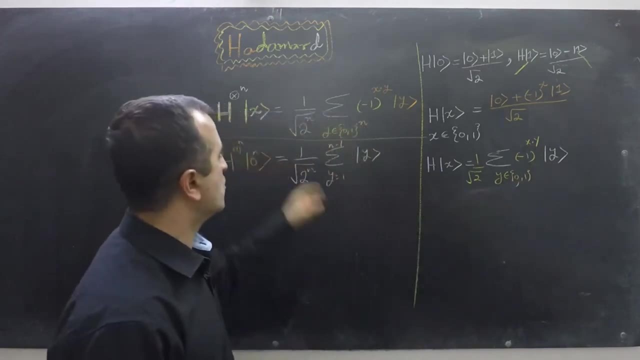 be minus 1 only when x and y both are 1, otherwise sine will be always plus. Now we're getting closer, because this formula here is starting to look more and more like this formula. We are not there yet, but this formula is almost like this formula. So let's say, I say this: 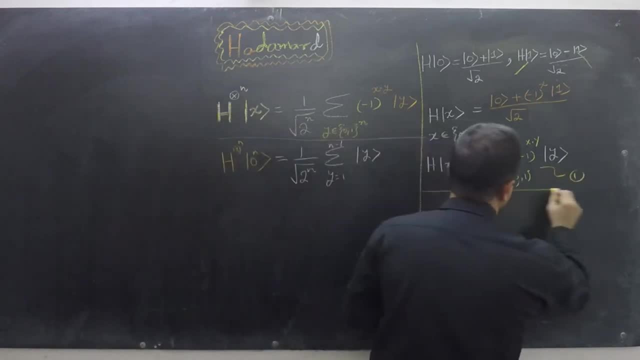 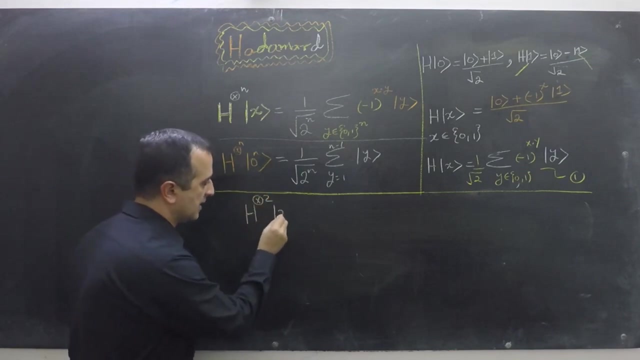 my equation 1, and now I continue. I have now general formula that works when x is single qubit. Now I have to write formula for 2 qubits. We say we apply Hadamard gate tensor product 2 on ket x where x is a 2-qubit register. 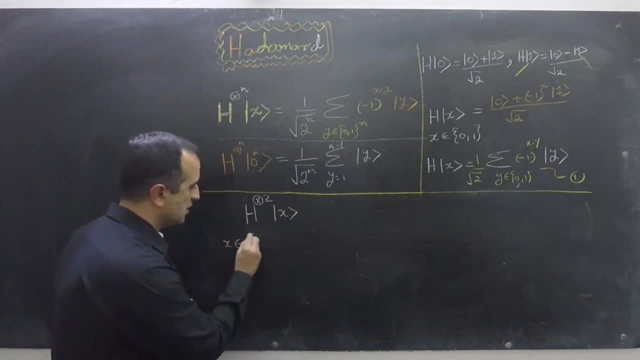 So we say that x belongs to 0,, 1, raised to power 2, which is equivalent to saying that x belongs to the set 0,, 0,, 0,, 0., 0, 1, 1, 0 and 1, 1. or we can also say that x belongs to the set 0, 1, 2, 3. so these three. 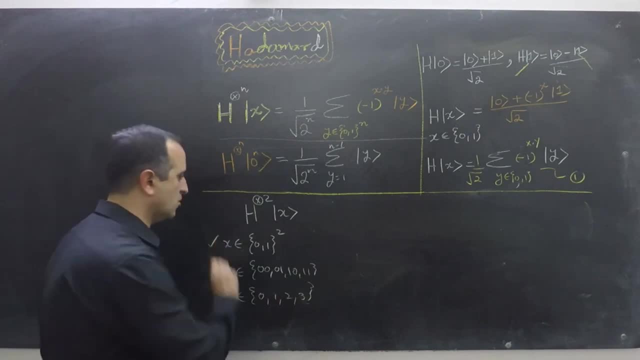 annotations are the same, but usually this one is used in quantum computing, so we will stick with this one for the time being. because it is two qubits, so you can write it like hadamard gate being applied on x 1, where x 1 is the first qubit of the register where x1 can take values. 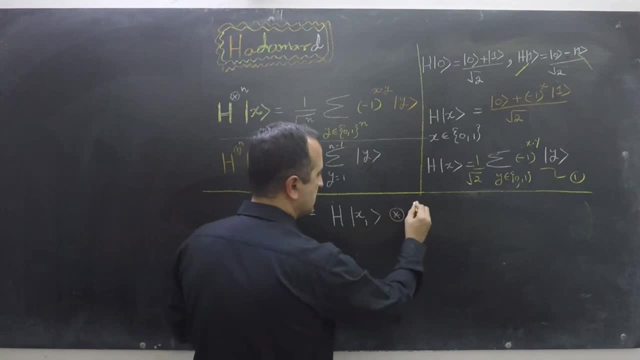 from 0 and 1 tensor product with hadamard gate being applied on x 2, where x 2 is once again a single qubit register. so these two are single qubit register. now we expand this equation by putting question number one here and here. so now we will have here question number one. 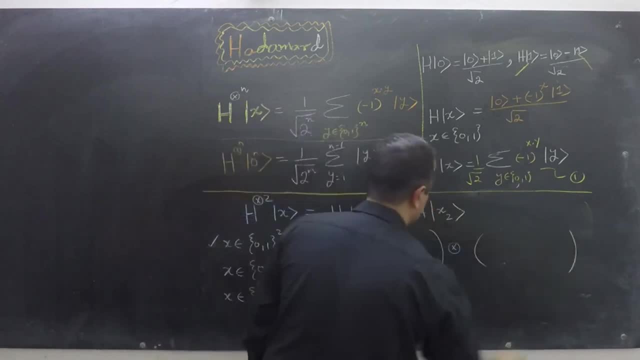 and we'll have the answer in the next section. i think so. now we extend this equation by putting question number one here and here. so now we will have here question number one and and tensor product with once again, equation number 1.. So we write here: 1 over square root of 2,. 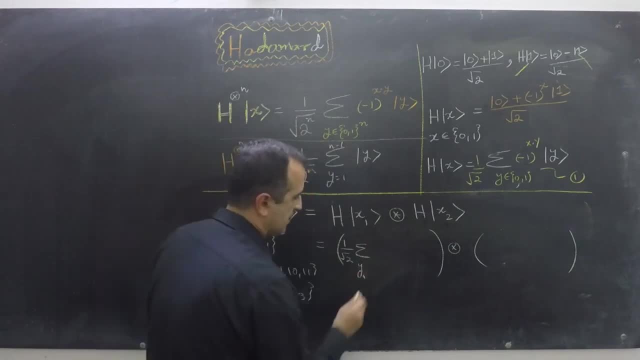 and now we have to introduce a new variable, y1, where y1 belongs to 0,, 1, and minus 1.. And because I have here x1 and I have here y1, so I say minus 1 raised to power x1, y1. 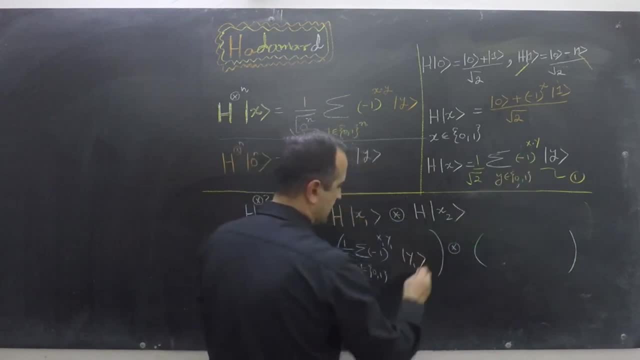 And similarly I have here ket y1.. This is my first equation. Second equation is going to be 1 over square root of 2, summation, and y2 belongs to 0 and 1.. y2 is my other variable and minus 1.. 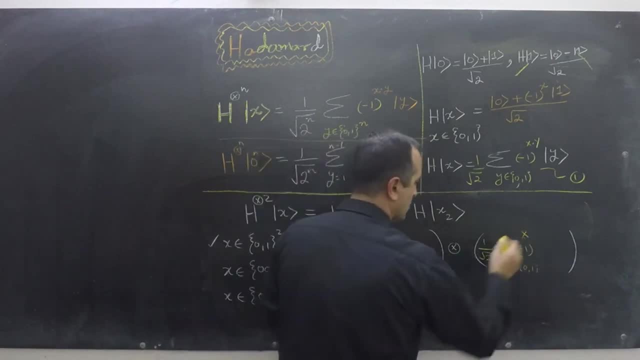 Now I will write here x2, because this is x2,, dot y2, and now I will say here ket y2.. So now we have to combine both of those equations. So now we have to combine both of those equations. So now we have to combine both of those equations. 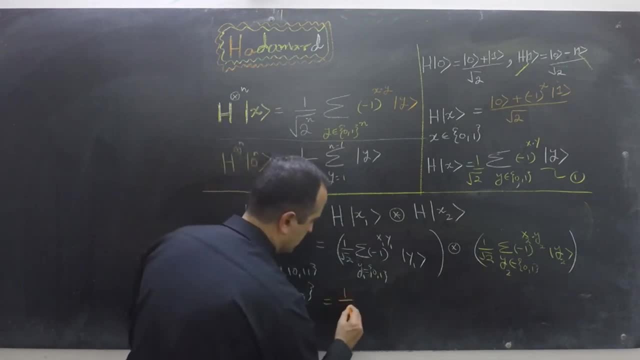 So what we have here is 1 over square root of 2 raised to power 2, because we have 2 times 1 over square root of 2, 1 over square root of 2.. So we have 1 over square root of 2 raised to power 2.. 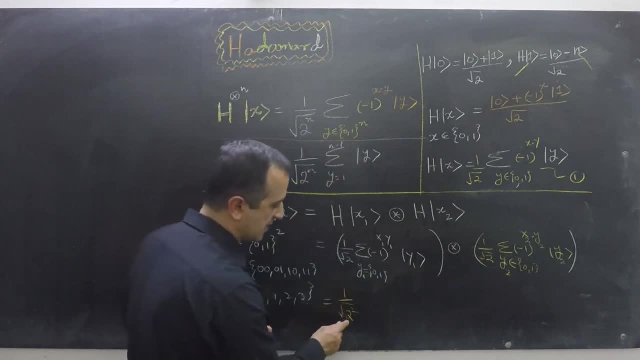 I could have written 1 over 2, but I'm writing it intentionally as 1 over square root of 2, raised to power 2, because from here we're going to get this equation eventually And then I will have here summation. 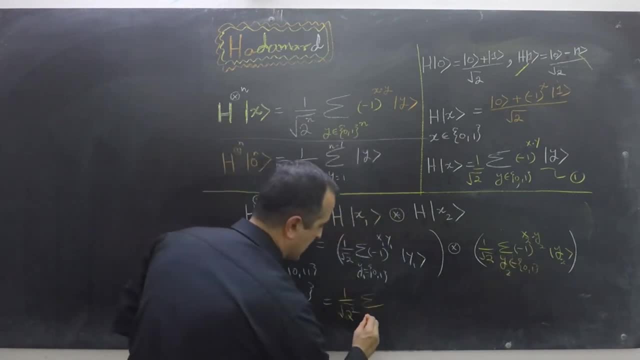 When we combine both of those summations we have a new variable, y. y will take value from 0,, 1, raised to power 2.. So you can think of both of those summations as for loop in computer science. 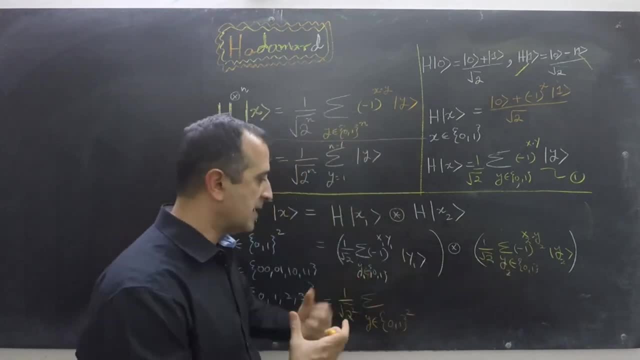 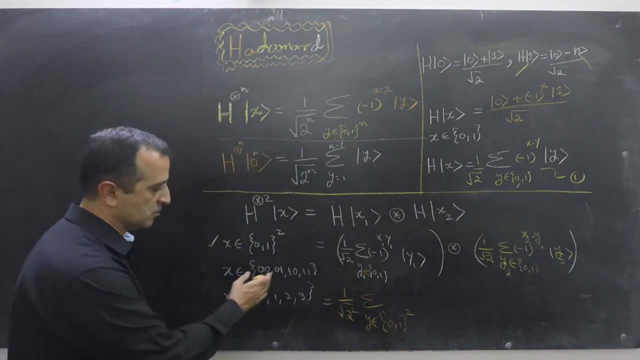 and they were nested for loop. So when we combine them we will have a loop that runs twice as many times. So y once again can take value from 0, 0, 0, 1, 1, 0, 1, 1.. 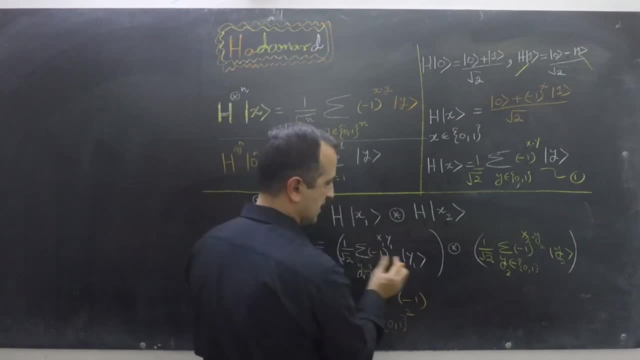 Then we will have here minus 1, because they are multiplying with each other, these two, These two numbers, so their power will add. we will have here x1, y1 plus x2, y2.. And then, because we have a new variable, y, so we will have here ket y. 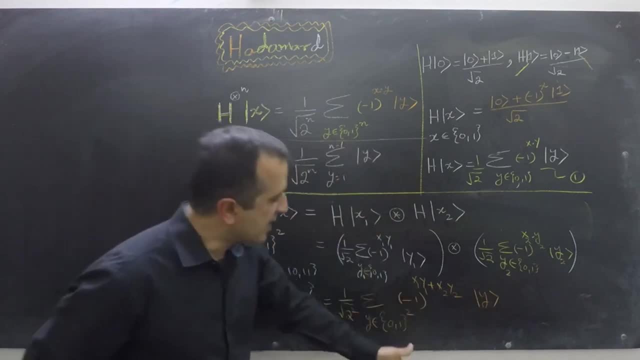 This is our new equation, And now we define x1 times y1 plus x2 times y2 as x dot y. So from here we get to this equation. This equation is also for the n-qubit, but this equation is just a general form of this equation. 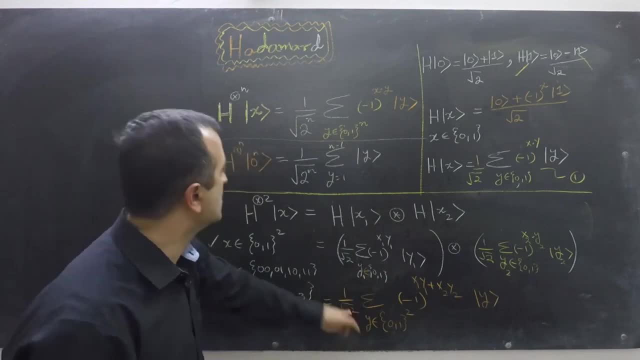 Here we have used two qubits, so we have say 2 raised to power 2.. Here we have n-qubit 2 raised to power n. So otherwise this equation is the same as this equation. Here we have y belongs to 0, 1 raised to power 2.. 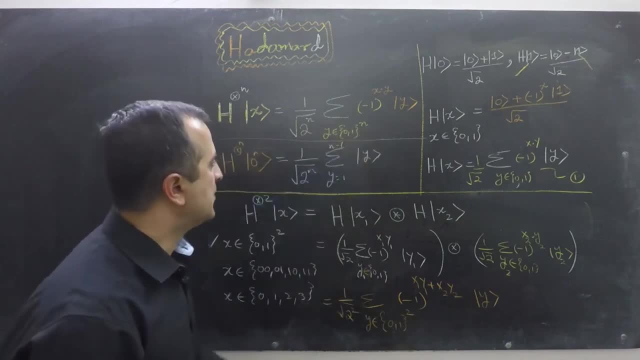 Here we have: y belongs to 0,, 1 raised to power n. But in quantum computing many times we only need to write this equation, Because in quantum computing many times we start with a register with all 0 qubits. 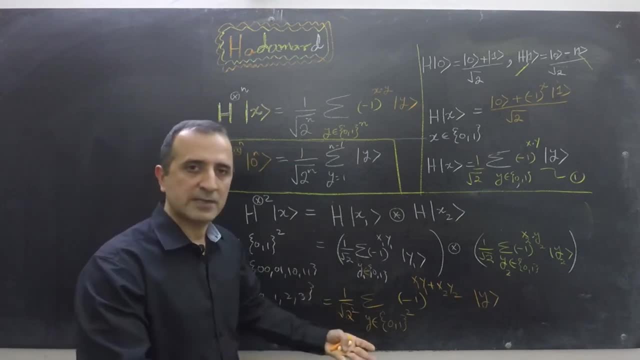 and then we apply Hadamard gate on that qubit When the register has all 0 qubits. then we don't have to worry about the sign, because the sign of all the terms is going to be positive. So that's why this one is a simplified version of this one. 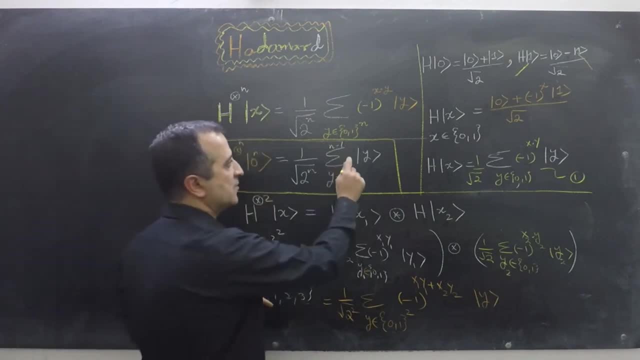 In this case we don't have to worry about the minus 1 sign here. I have here used a different notation, that y from 1 to n minus 1, but this is the same as saying y belongs to 0,, 1 raised to power n. 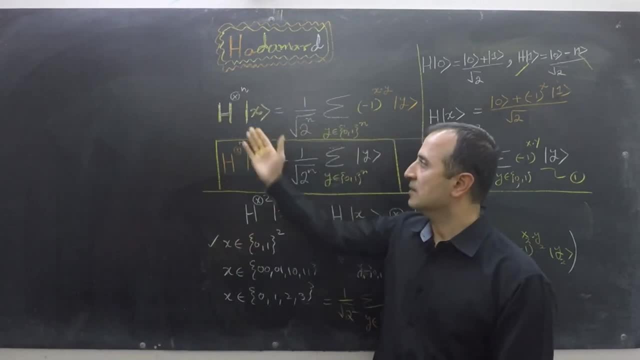 So I hope that now you'll be able to understand these equations and can expand these equations, And whenever we are developing a quantum algorithm and we apply Hadamard gate on some qubits and we just quickly write this equation, then you will not be confused and you know what's. 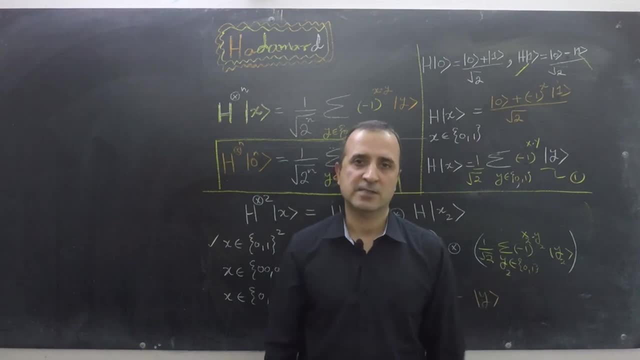 going on. That's it for this video. See you next time. Stay tuned.